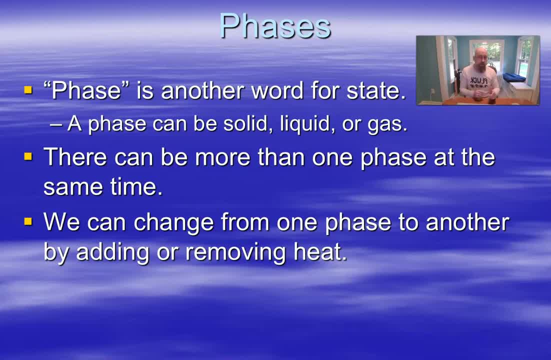 to matter, that is in one of solid, liquid or gas, right, And so, like ice is in the solid state, Water is in the liquid state, Steam is in the gas or vapor state. The word vapor and gas are interchangeable. in this case, Phase can also be solid, liquid or gas, but there can. 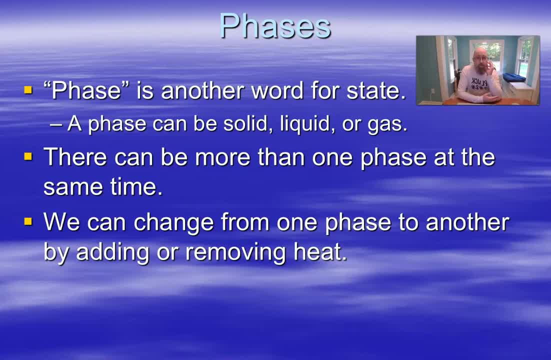 be more than one, And so that's an important thing to understand. Phases can mean parts of a larger group of things, So, for example, there could be a mixture. If I put sand in water, there would be two phases present: There would be the solid sand phase and then there would be the solid water, And so 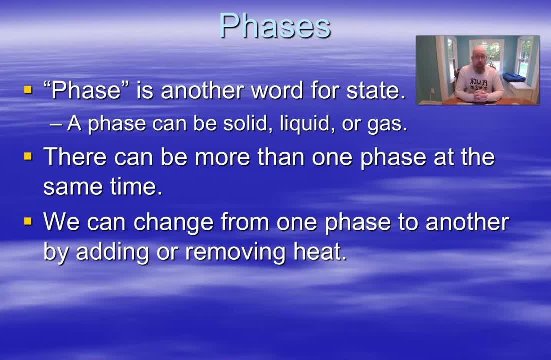 the liquid water phase, right, And so we don't describe those as states who use phases. Phase can also be more complex later on in the year and we'll talk about that when we come across it. In this case, we're talking about phase changes, which could also be called changes of state or 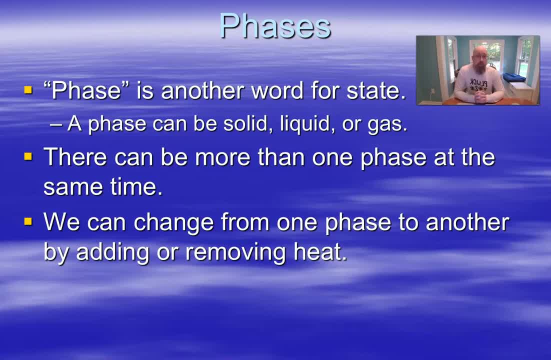 state changes. But the reason why I'm using the word phase here is because when there's a phase change, there is more than one state present at the time. So, for example, when I melt ice, there's both solid and liquid. The ice gets wet while it melts. When we boil water, there is both. 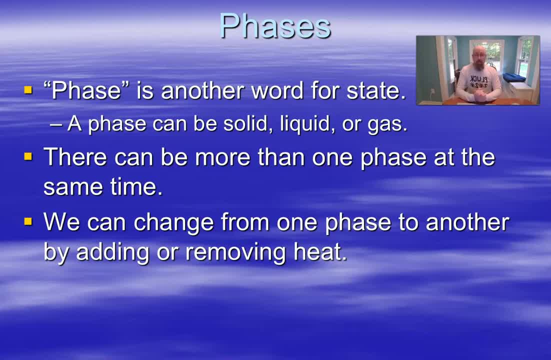 liquid and gas. The bubbles are the gas phase, And so we have more than one phase during a phase change. And when we change phase, of course energy is directly related. I could be adding energy to change phase, or I could also be removing or cooling something down to change phase. 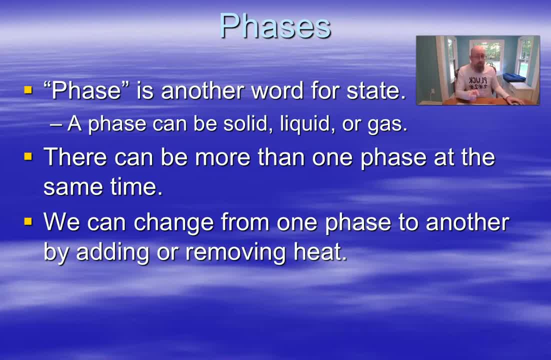 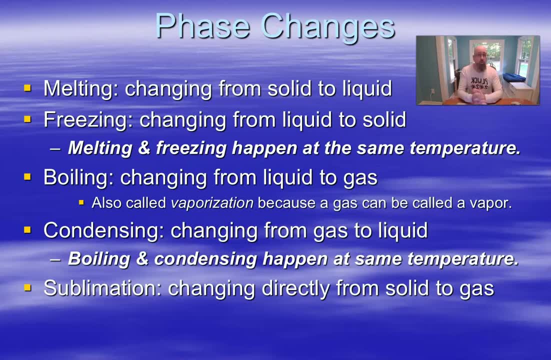 But, as we learned in the lab, when we're changing phase, the temperature stays the same, And that's something that we're going to talk about in a little bit. So we're going to talk about the changes that we're going to discuss and draw out as we go forward. Now, first, a quick review. I'm 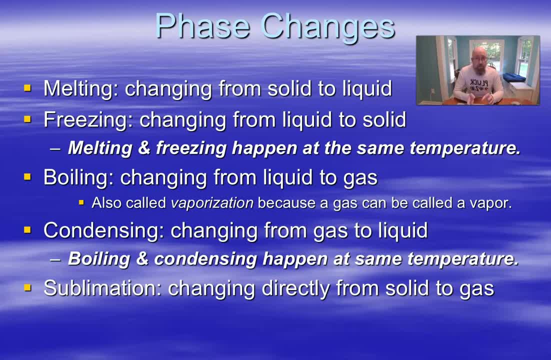 sure you know all these terms, But when we're talking about changing from solid to liquid or from liquid to solid, we're talking about melting and freezing. Now I want to make the point that the melting temperature is the same as the freezing temperature. We call them the melting. 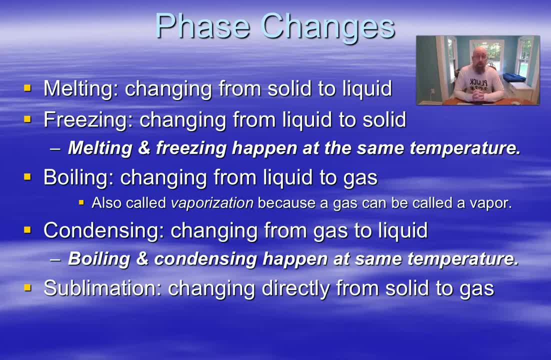 point and freezing point, or just the melting point. sometimes There's a deeper name for that that will come up in one of your packets as well. Melting and freezing happen at the same temperature. So if we're talking about whether something will freeze over on a roadway, for example, 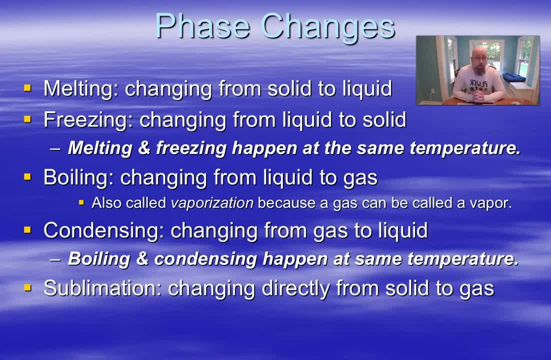 so we're talking about 32 degrees Fahrenheit. will it cool down below 32 degrees Fahrenheit or zero Celsius? Same thing: if we have snow and we're asking whether it would melt right, Will it warm up to 32 degrees Fahrenheit or zero degrees Celsius? And so it just matters what direction. 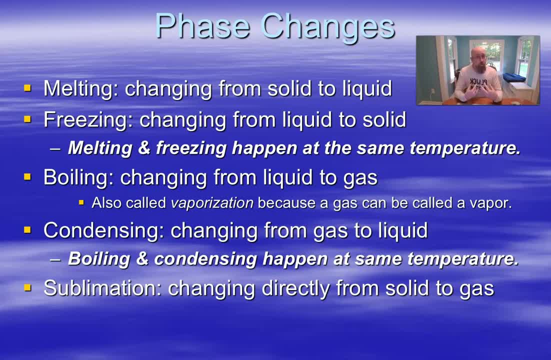 you're going, Are you adding heat which is melting or are you removing heat which is freezing? But they happen at the same temperature. It's important to understand that. Same thing for boiling and condensing. Boiling and condensing happen at the same. 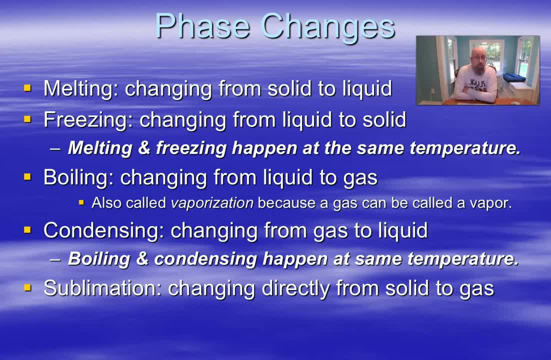 temperature. 100 degrees Celsius or 212 degrees Fahrenheit are those temperatures. If I'm adding heat, of course I'm boiling, and if I'm removing it then I'm condensing. Boiling can also be called vaporization, right, Just like gas phase and vapor phase are. 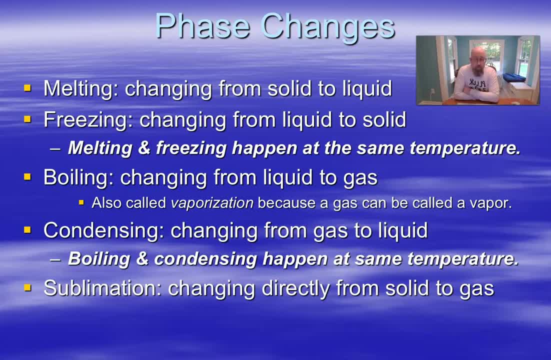 interchangeable. boiling and vaporization are interchangeable, But evaporation is something different that we're not going to talk about right here. So evaporation can happen at any temperature, but vaporization only happens at one specific temperature, which is the boiling point temperature, right? So just like melting and freezing happen, 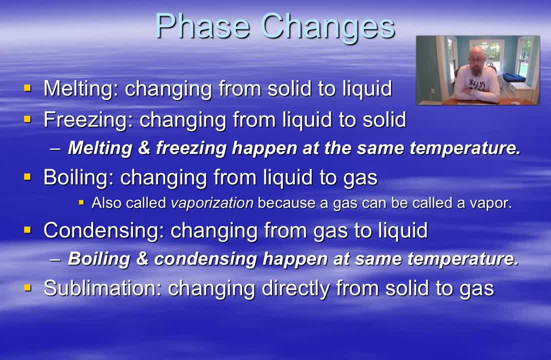 at the same temperature. boiling and condensing also happen at the same temperature. That's why, over a stove, if you're boiling water, you often have both boiling and condensing, especially if you have the lid on right, And so the steam comes up from the water. 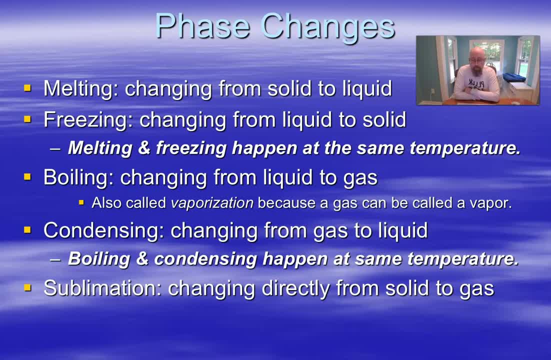 hits the lid and it condenses and drips back down inside there. Now there are phase changes to these, So sublimation- you can actually change directly from a solid to gas. Dry ice is the most famous thing that sublimates and that's because it doesn't go through the liquid phase, so it never 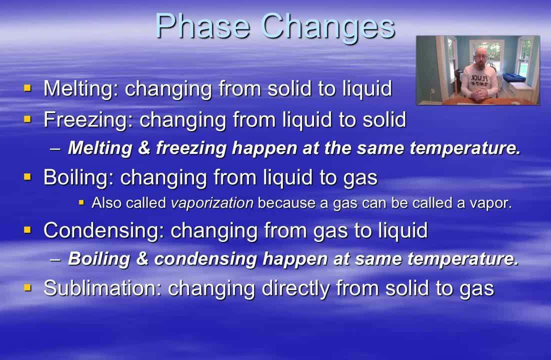 gets wet, It turns directly from a solid to a gas. Great for shipping frozen things because it won't make your package all soggy and ruin everything. There is an opposite to sublimation, but it almost never comes up so I didn't put it in these notes. But the opposite is deposition, something that 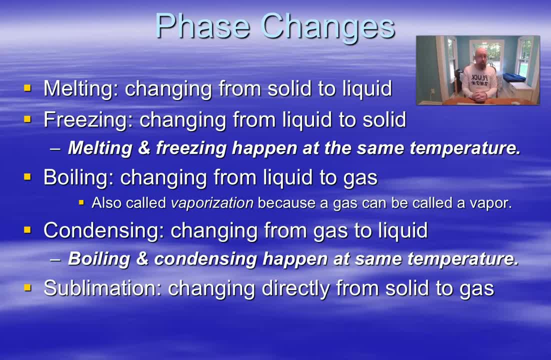 changes directly from a gas to a solid. There are some pollutants that can deposit and there are some pollutants that can deposit on substances. So just like dew forms on your car when moisture condenses out of the air around you, so can some pollutants form as a solid powder on a car. 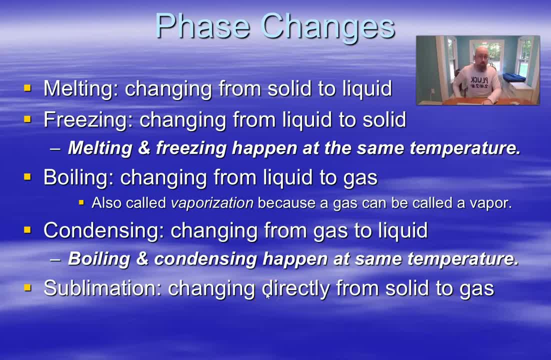 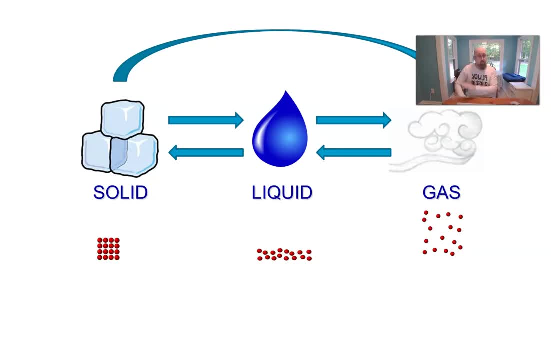 for example when they deposit. But sublimation is a much more common encounter. of this Quick visual just to review that and connect with the visuals that I gave you on Monday in class. The solid with its rigid structure, geometric often. solids often have geometric structures. The liquid with its still close together particles, but yet 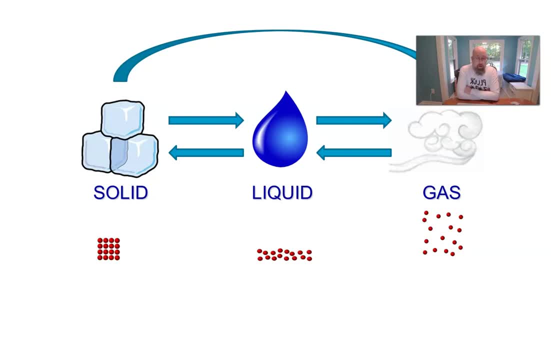 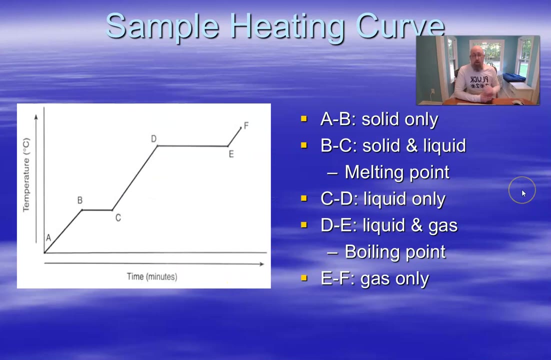 free to move, and so no defined shape. And then the gas with spread out particles, And this diagram doesn't do it justice. The particles of the gas would be more spread out than that, And then this overarching arrow here would represent sublimation, a solid going directly to gas. Now there's a better. 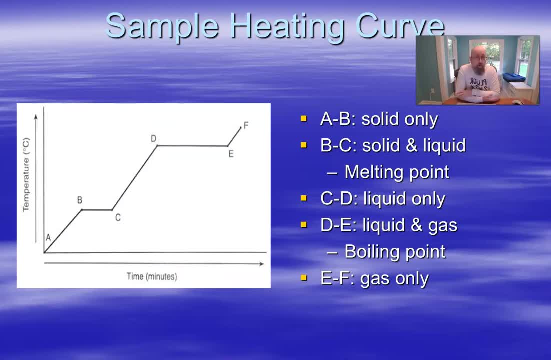 way to represent all of these phase changes and we can actually put them on a graph, right, And this is similar to the phase changes that we've seen in the past, So we can actually put them on a graph, similar to the graphs that you made in your lab, except you did two separate graphs and they both 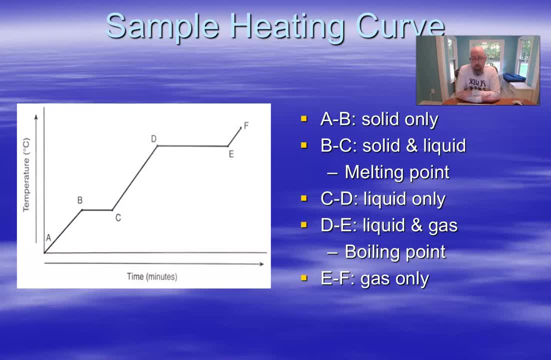 related to a single phase change. In this particular case, we've got one substance and we're going to go through both phase changes, right? And so let's talk a little bit about what this represents. We can do this for any substance. Every substance has a heating curve and it will have the same 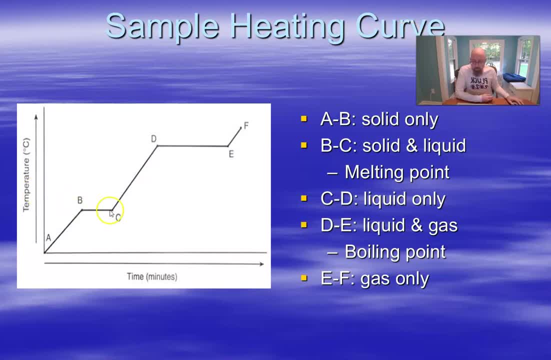 general shape. Some of the details might change, like the particular temperatures of these flat spots here, or particular temperatures of these flat spots here, or particular temperatures of these plateaus. The slopes of the lines might change, but otherwise the overall shape of this would be. 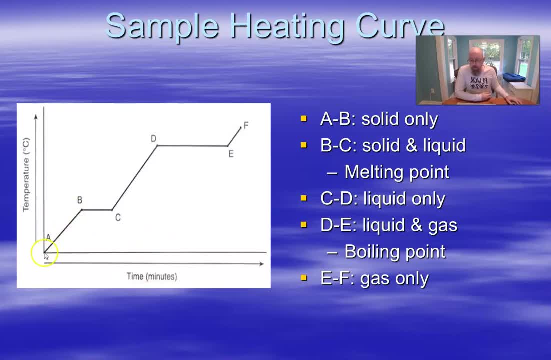 the same for any substance. All right. so when we start out at the lowest temperature, temperatures on the y-axis here right. So as we go vertically we're increasing temperature. As we start out at the lowest temperature, here we have a solid phase, right, Or solid state if you prefer that term. 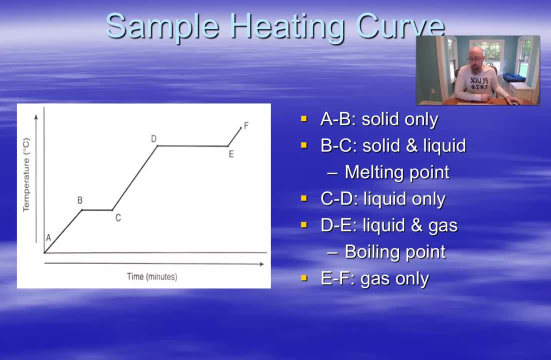 Solids always occur at the lowest temperature because they have the lowest kinetic energy right, And so if something starts out as a solid, then in order, before it starts out as a solid, before I can even melt it, I have to get it up to the melting temperature. A lot of people don't. 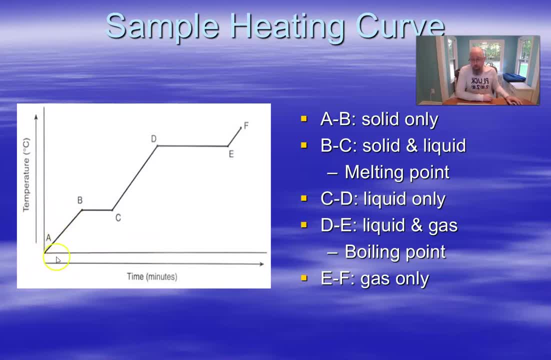 realize this, but when you pull ice out of the freezer, the freezer is usually below zero degrees Celsius, sometimes as low as negative 10, right. Then the ice is solid in there and until you warm it up to zero degrees Celsius it won't actually start to melt. Now that happens almost. 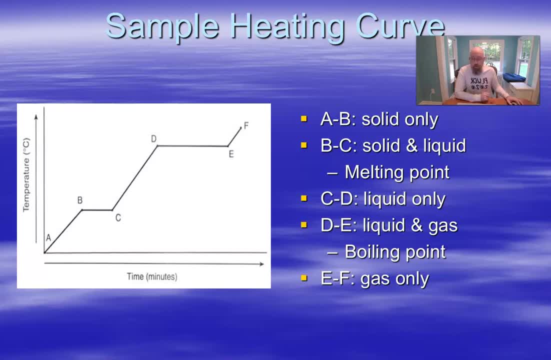 instantly if you touch it, because your body warms up the surface layer of it. But if you leave ice out on a cold day, it won't actually start to melt. So when you pull ice out of the freezer, it won't immediately become wet. It has to warm up just a little bit before it starts melting. right And so? 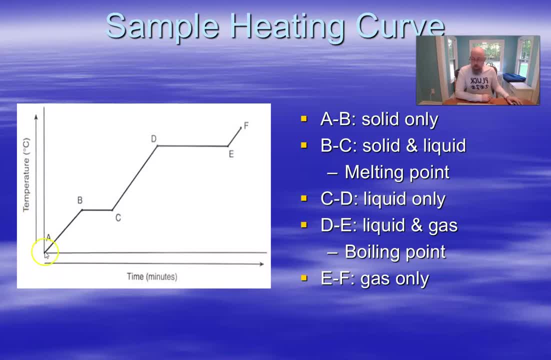 we are warming up from. whatever temperature we're starting at doesn't matter until we reach the melting point. temperature right AB means we have only the solid. Then, as we saw in the labs, the temperature remains constant during the phase change, which we'll talk about a little bit more. 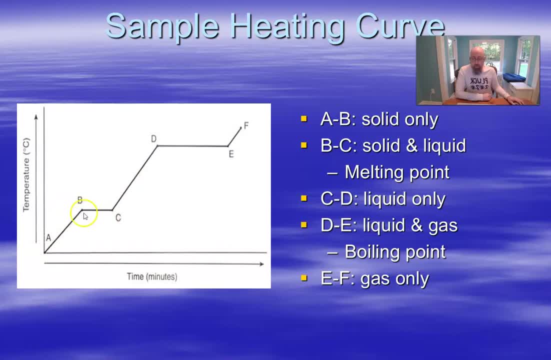 in just a moment. So we're warming up from whatever temperature we're starting at until we reach the moment right. So the temperature remains constant means that this is a flat spot. right here, This flat spot represents melting. The melting process happens as we go from B to C, So over time, as I 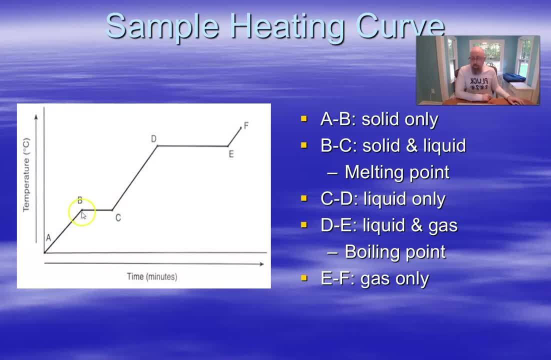 continue to put heat into this. we didn't stop heating this, but the temperature stopped changing, and that's the sign of a true phase change. The temperature remains the same throughout that, So BC represents the change of solid to liquid, which means both of them are present at the same. 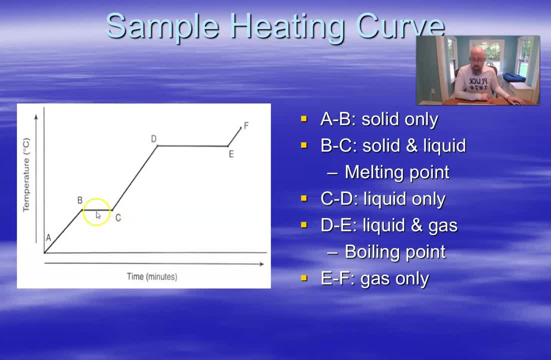 time, Right, That is what the melting point is. If I take this line and trace it back to the temperature axis, the y-axis, it will tell me what the melting point temperature is, And that's something you can do in your lab. is read that off of your graph, right? So then, once we get to C, it means that 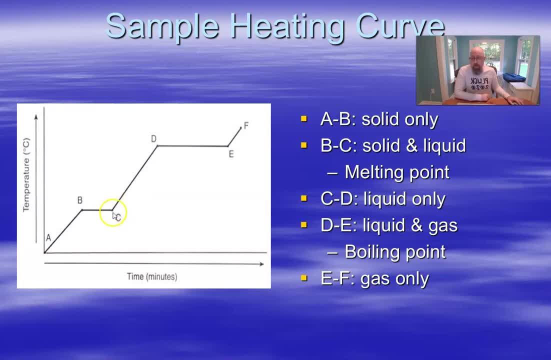 all of the solid has been melted and has turned into liquid, and then the liquid can begin to rise again. Now, in reality, that's kind of a simplified version of thinking about it, because in reality, as soon as some of it melts, it's going to start to rise again. So that's what we're. 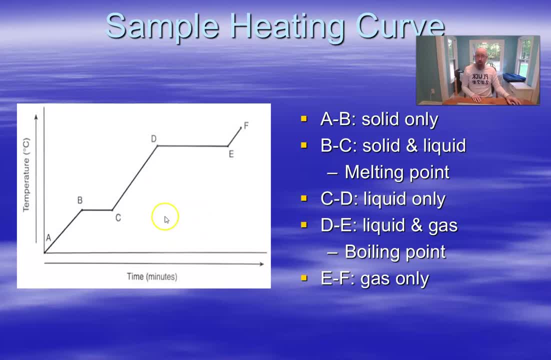 going to do? We're going to wait for all of it to turn to liquid, and that can actually complicate things. We have a little problem with that in part two of the lab. It's difficult to get the temperature of the solid, and so instead you have the temperature of the liquid, and because of that, 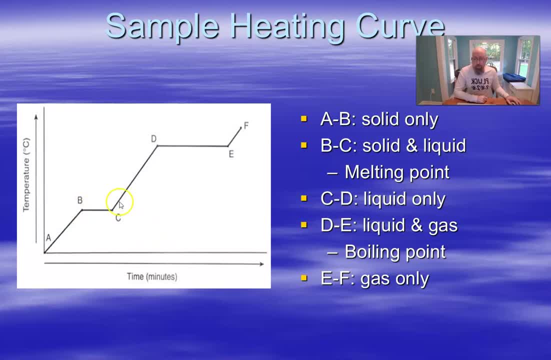 it screws up the data just a little bit. It makes it harder to spot this flat spot. Now, with boiling, though, it was very clear, Right? So when we get to this point, we have all liquid, right? So Cd represents liquid, and it might be a good idea for you to sketch out a graph like this. 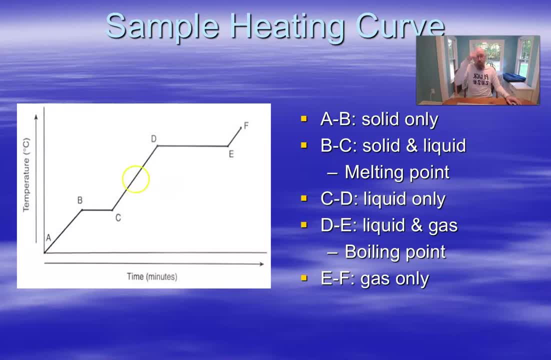 and label these, and there's also going to be other pieces of information that we're going to attach to this be a real useful study guide. to have a sample heating curve like this right- So Cd here represents liquid right. During the liquid state, the temperature can rise again. 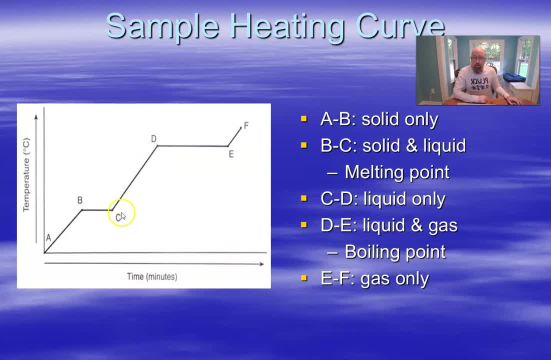 because there's only one state present. okay. And then finally, eventually, the liquid is going to reach its boiling point. okay, At its boiling point again, the temperature is going to rise again. The temperature is constant, which we saw very clearly from part one of the lab During the 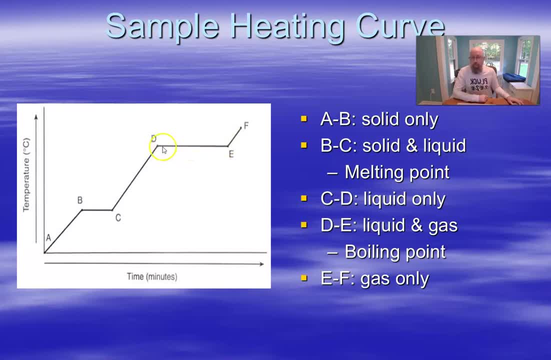 boiling process. the temperature remains the same even though we're still putting heat into it, right. And so, from D to E, we have both liquid and gas. We have the liquid boiling, creating gas bubbles that are within there And again, if I trace this back to the y-axis, I can read off: 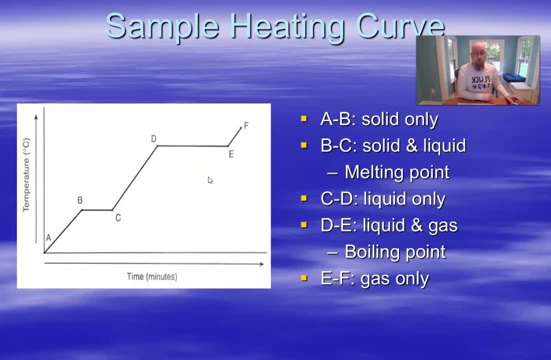 the temperature if the y-axis was labeled the temperature at which boiling happens or the boiling point temperature, right? So we have three sloped segments and we have a temperature of 0.0t in that acceptance. so 3.0t over here And notice that it's 3.5t in the bottom of that. 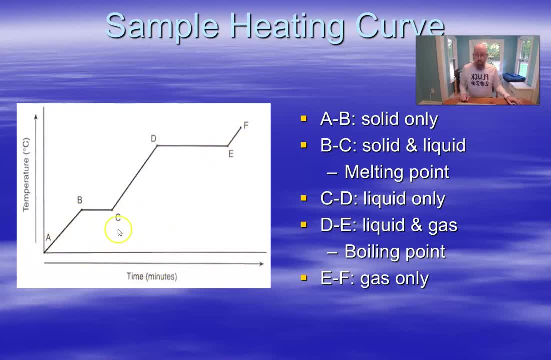 climate. Now we're measuring six trying stop over. Formally that means 3.4t, 12 tenha A, b, d e, f. Those represent the three states of matter, solid liquid gas In between themwe. 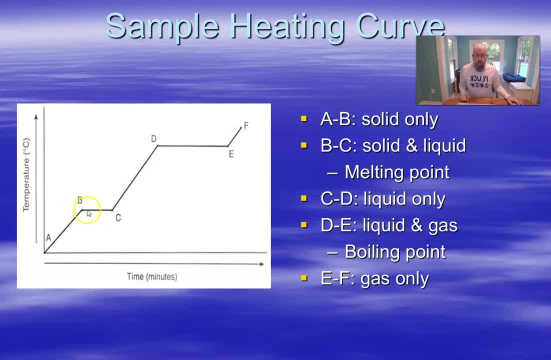 have flat spots with zero slope. The lower flat spot is the melting point and the upper flat spot is the boiling point. So the flat spots represent phase changes and the sloped lines represent single states along the way. So why does this happen? Well, when we have a solid, rigidly. 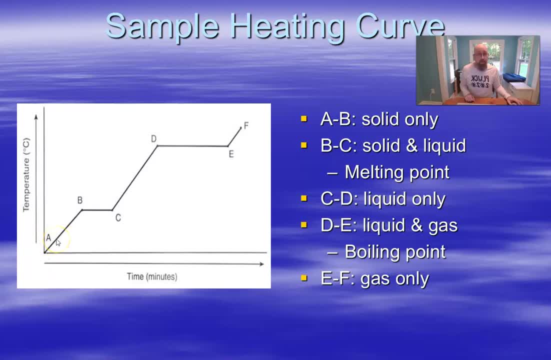 packed together and some of its particles are large. they measured the sort of landlocking of the body from the summer to the evening has not been seen, so they're oriented at f. we've found that the different states are tightly fit and in a specific structure. as I raise the temperature they're going to speed up. 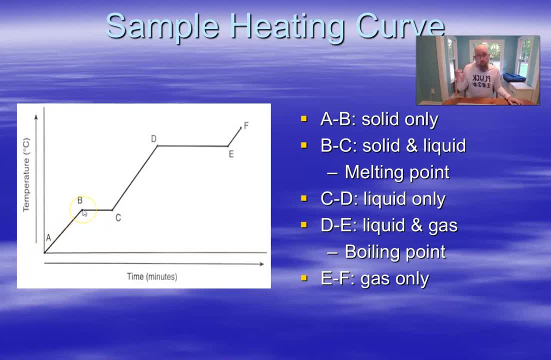 They're going to vibrate more and more. At some point they will actually break loose from the structure. In other words, they're vibrating too much. There's too much kinetic energy in them to remain within the limitations of their structure. So when they break out, then they 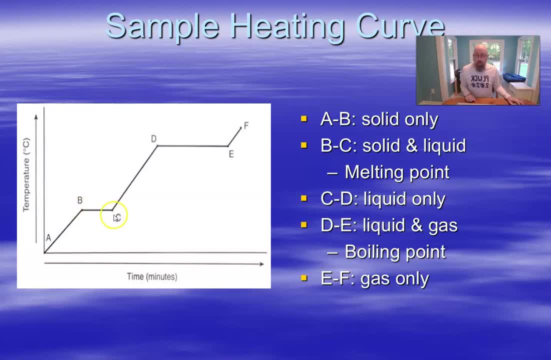 begin to turn to a liquid, and that's the melting process. right here, The rearrangement of the particles, breaking apart that structure and allowing them more freedom to move, is what's going on there. Same thing with the liquid. Once we get here, we're in the liquid state. 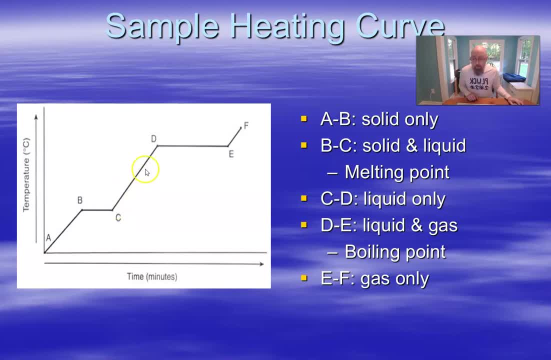 but the particles are still crowded close to each other And as I speed them up by raising the temperature, increasing their kinetic energy, they'll vibrate faster and move faster And eventually they can't move any faster without separating from each other. They've gone as fast. 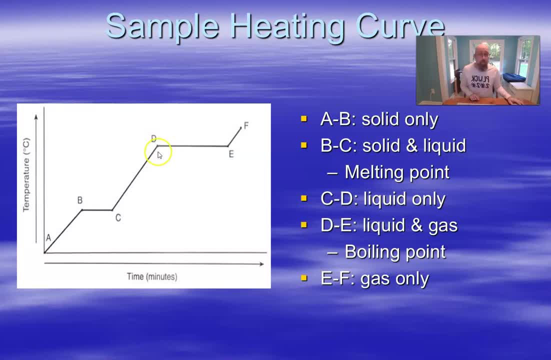 or they're going as fast as the crowded nature of those particles will allow, And so because of that, they need to convert to the gas state. That's what happens here: The particles are pulled apart from each other, So it's again a rearrangement, but it's a different kind of rearrangement. 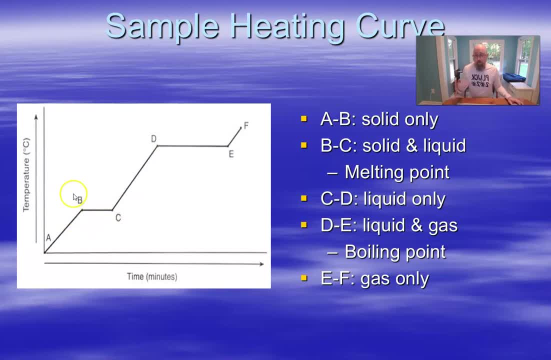 Here the solid structure is being broken apart, allowing the individual particles to move separately. Here the individual particles are actually being separated from each other, increasing the distance so that they can move independently of each other without having to worry about bumping into each other, And eventually we get to the gas, And I should 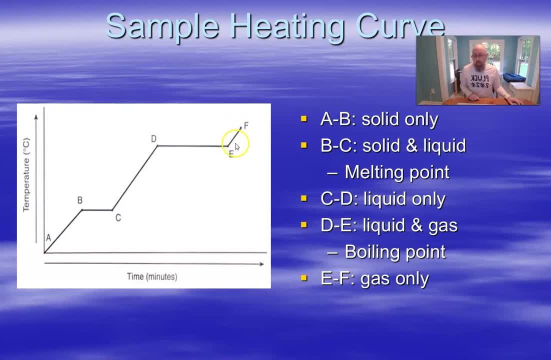 point out that the gas is not going to move as fast as the crowded nature of those particles. I should point out that this should have like an arrow on it here, because in reality, for most materials, you can continue to heat the gas and its temperature will continue to rise. 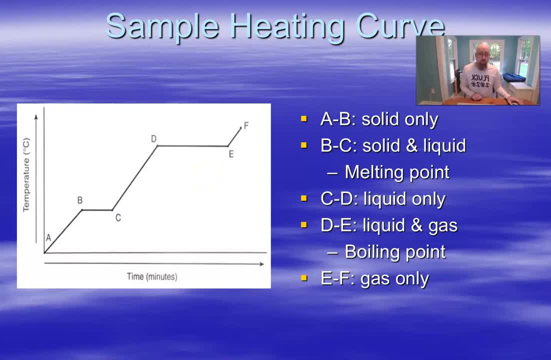 without any real limitation. The only reason why that wouldn't be true is if, at a certain temperature, the chemical breaks down or decomposes, which can happen to some chemicals. All right, so that's the breakdown of the heating curve. Go back and reference that if you need to. 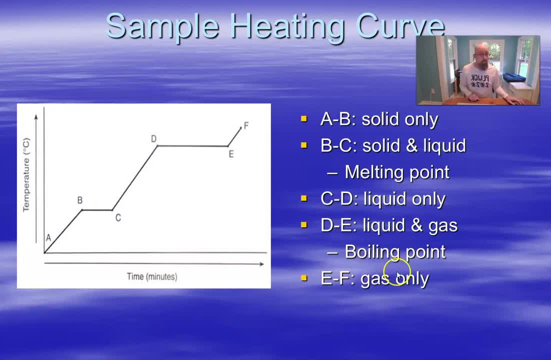 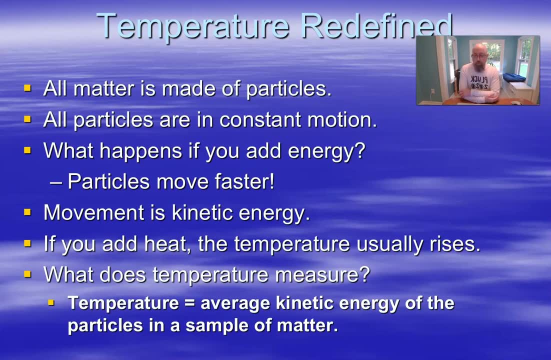 and draw yourself a nice little study guide, because you're going to need that for the practice that we're going to be doing next. So let's go ahead and start. All right, so a quick review of our new definition of temperature. All matter is made of particles. 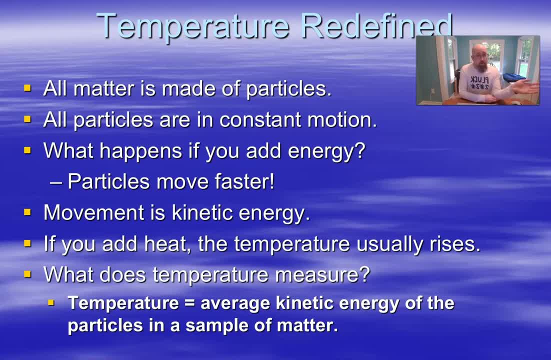 which are in constant motion. If I add energy, they move faster right And so faster speed means more kinetic energy. So when I heat up a particle, then they move faster and the temperature rises. So that means that temperature is actually measuring the speed of movement of the particles. 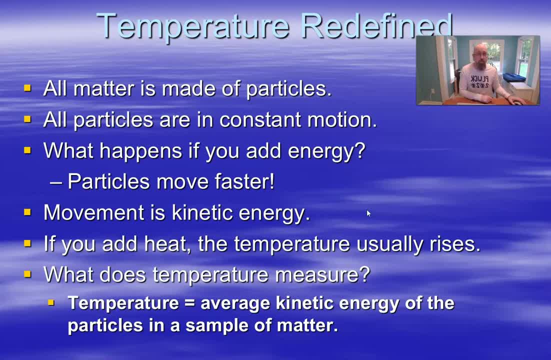 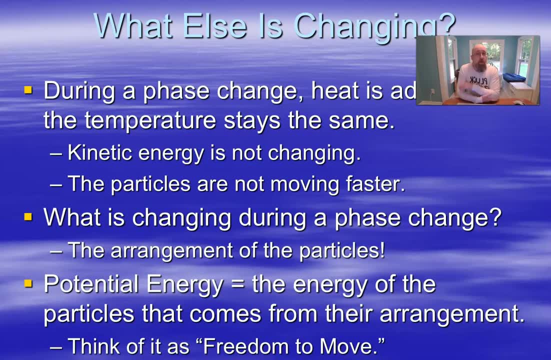 the average kinetic energy. So that's what one of the things that we talked about in class on Monday. Now let's talk about the other kind of energy. So during a phase change, even though we're adding heat, the temperature remains the same. All right if temperature is. 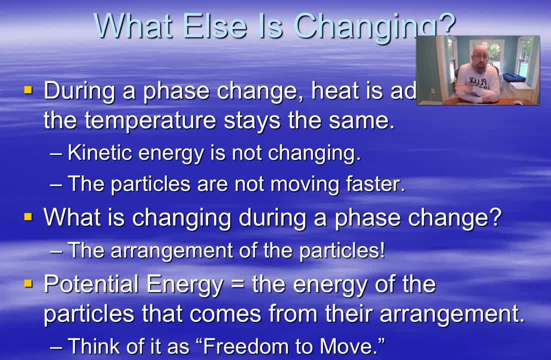 kinetic energy, then that means the kinetic energy is not changing during a phase change. right: Temperature reflects kinetic energy. Temperature remains the same during a phase change. So therefore the kinetic energy remains the same during a phase change. So that's really important. We're putting energy into 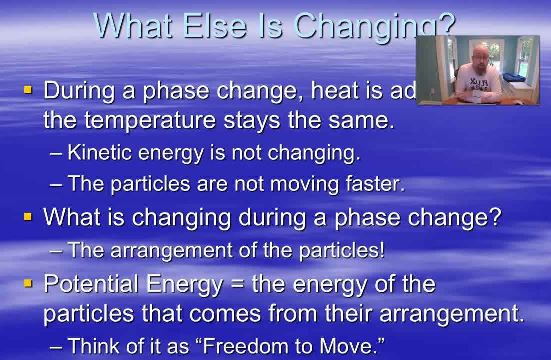 the substance, but the kinetic energy of the substance is not changing. Then what's left? Well, there's only two broad types of energy. If it's not kinetic energy, then we must be increasing potential energy within the sample. okay, So potential energy. 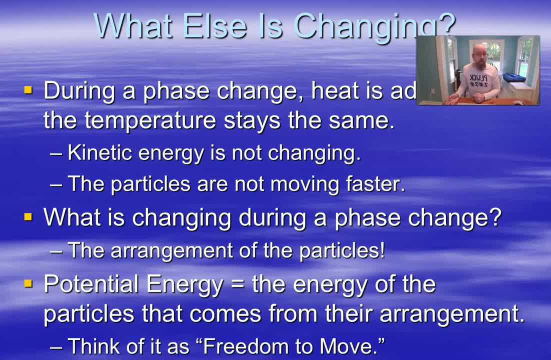 which is stored energy has to do with the arrangement of the particles. okay, That has to do, in simple terms, with freedom of movement. So think of the potential energy of the particles as the energy of the particle. So if we're adding energy to the particle, then we're increasing. 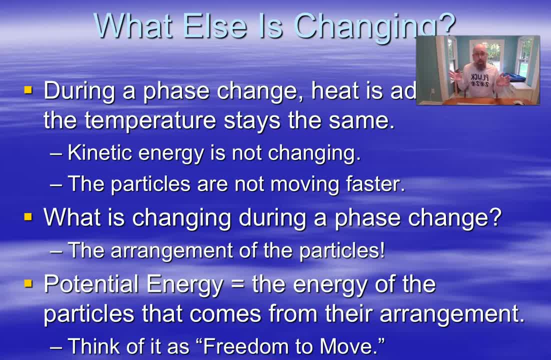 their freedom of movement. right When I have a solid, they're packed really tightly together and held rigidly in place by strong forces which we'll discuss later in the year. So there's not a lot of potential for movement, There's not a lot of possibility for the particles to move In order. 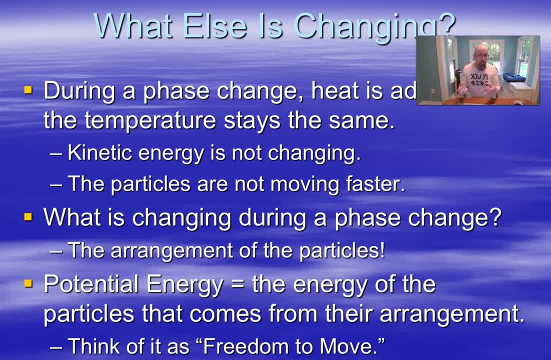 to give them more potential to move, I have to break apart that structure and free the individual particles so they can move around each other more. When I do that, that's a phase change, changing solid to liquid. During that time I have to break apart the structure and free the. 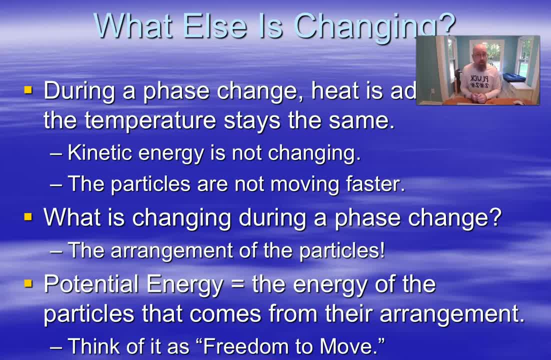 individual particles. During that time, the temperature doesn't change because the kinetic energy is not changing. Instead, the heat is going into potential energy. It's going into rearranging the substance Again. whenever there is energy involved, there's going to be something. 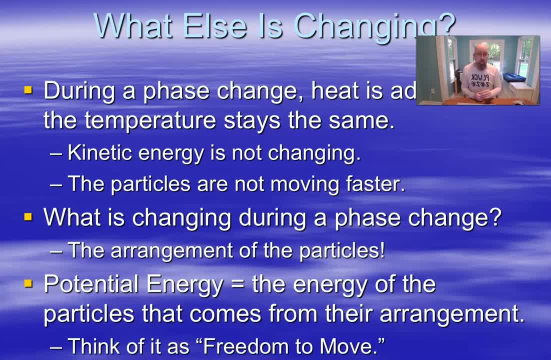 changing, but in this case it's the arrangement of the substance During the phase change. the arrangement of the particles is changing, not the speed of movement of the particles, right, So potential energy increases during the phase change, right. And 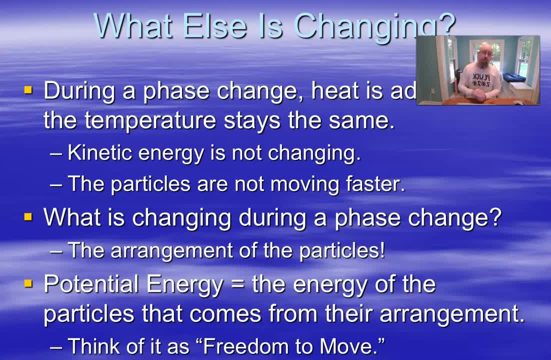 once the phase change has been completed, then kinetic energy can begin increasing again. Same thing happens when we get to the next phase change, right? So each phase change represents a change of potential energy, while the slope lines represent primarily a change in kinetic energy.